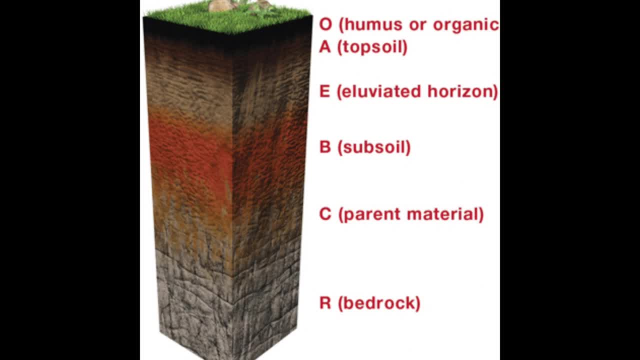 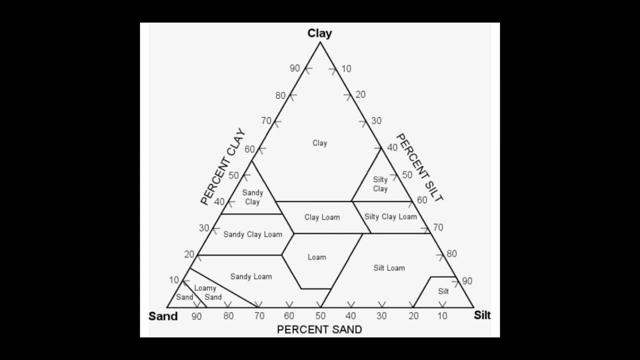 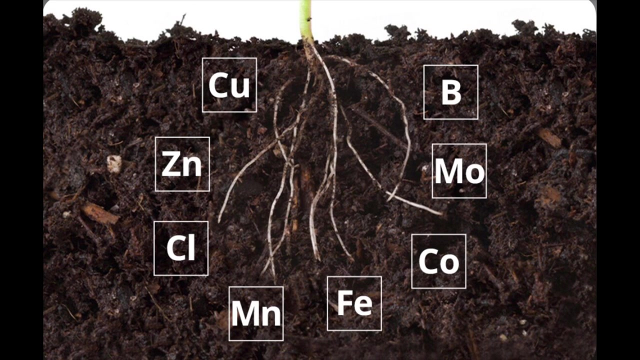 parent material And R is the bedrock level. A good tool to use to determine the soil type is a ternary diagram. Ternary diagrams classify soils by their sand, silt and clay content. When soil types are categorised, there are two categories Where there are No 2 seeds. 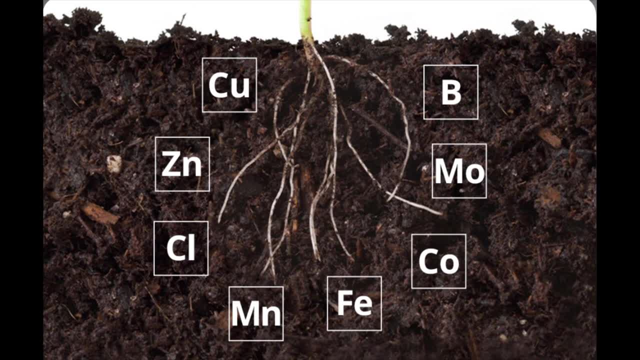 there is a No 3 seed or No 4 seed type for which soil type is going? Thanks for listening. 識 includes carbon, hydrogen and oxygen. The solid soils category includes nitrogen, phosphorus, potassium, calcium, magnesium and sulfur, Both the air, water and solid. 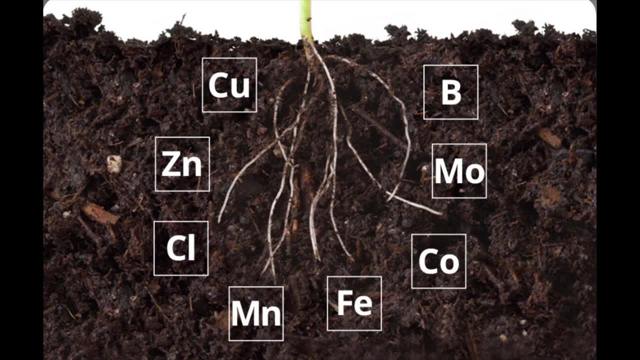 soil categories are part of macronutrients. The micronutrients include iron, manganese, boron, zinc, chloride, cobalt, molybdenum and nickel. Let's move on to the functions of soil. Soils perform six key functions in the 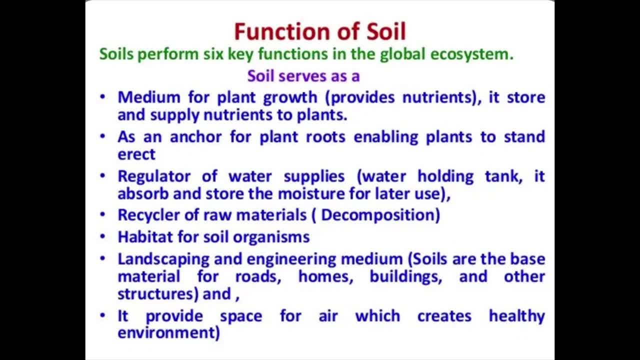 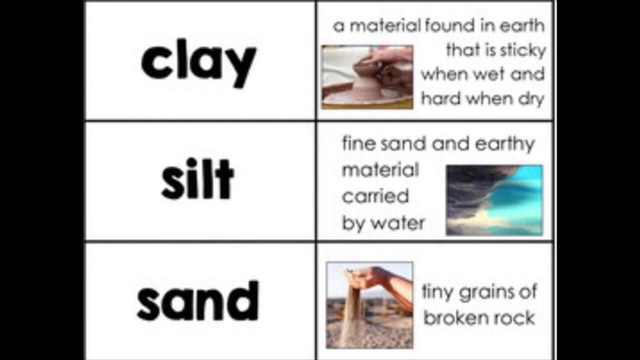 global ecosystem. Soil serves as a medium for plant growth, an anchor for plant roots, a regulator of water supplies, a regulator of raw materials and a habitat for soil organisms, landscaping and provides space for air. Now let's move on to some important vocabulary. Clay is a material found in earth that is sticky. 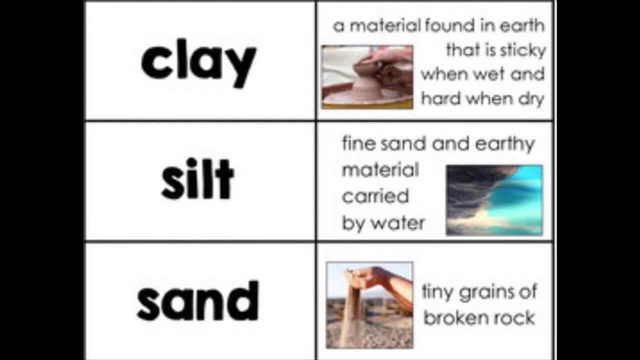 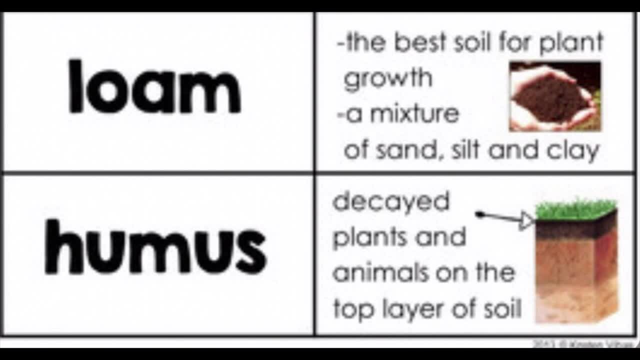 when wet and hard when dry. Silt is fine sand and earthy material carried by water, and sand is tiny grains of broken rock. Loam is the best soil for plant growth and it's a mixture of sand, silt and clay. 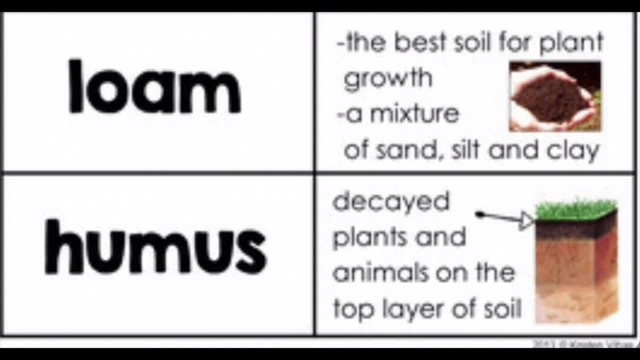 Humus is the best soil for plant growth and it's a mixture of sand, silt and clay. Humus is the best soil for plant growth and it's a mixture of sand, silt and clay. Humus is decayed plants and animals on the top layer of soil. Topsoil is the top. 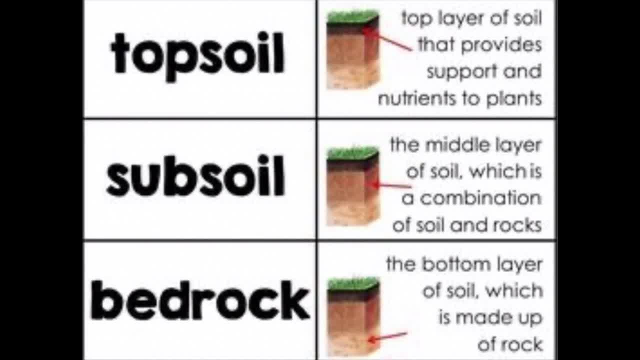 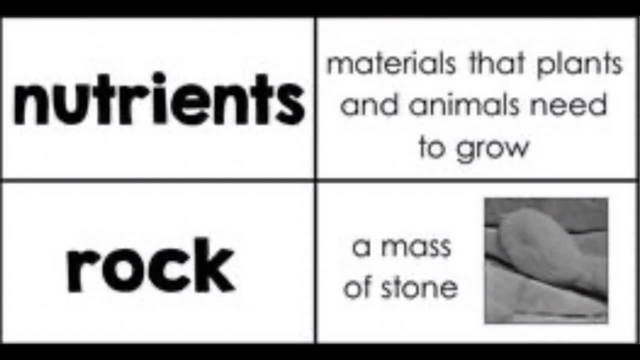 layer of soil that provides support and nutrients to plants. Subsoil is the middle layer of soil, which is a combination of soil and rocks. Bedrock is the bottom of soil, which is made up of a rock. Nutrients are materials that plants.